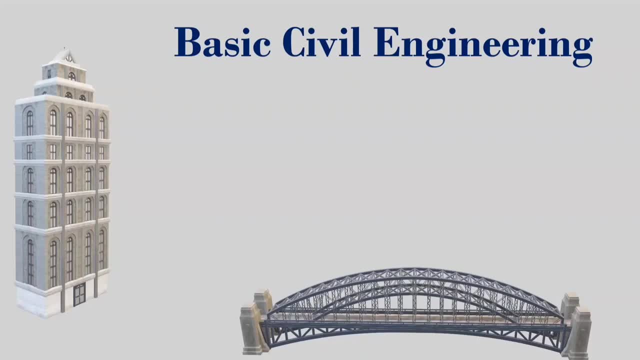 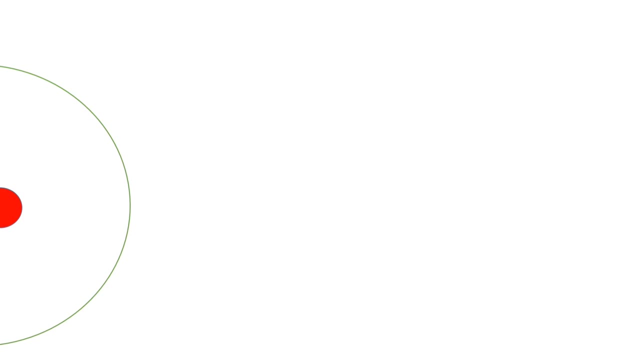 Hello students, Welcome to the lecture series of basic civil engineering. In this lecture we are going to learn about introduction of this subject. So let us start with introduction of basic civil engineering. We will start with outline of this session. First we will see about what is engineering, Then we will learn about what is civil engineering. After that we will see different branches of civil engineering And then we will learn about scope of civil engineering. 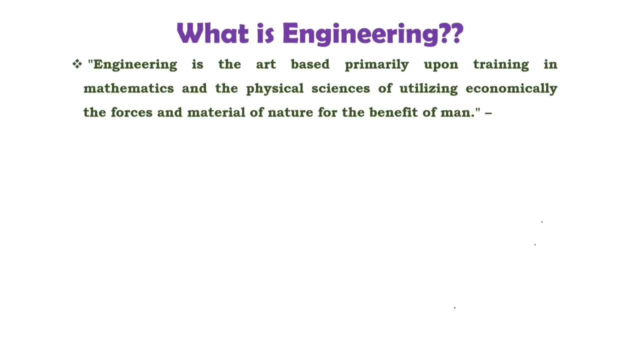 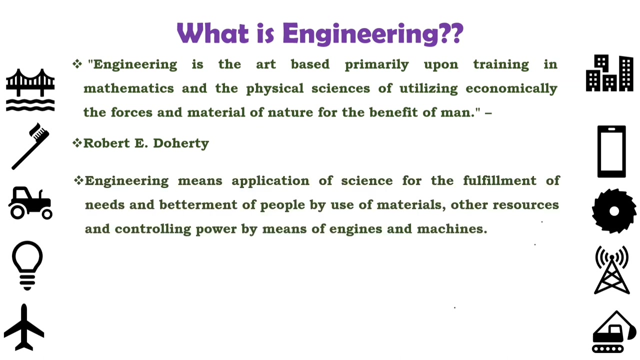 So let us start with what is engineering? Engineering is the art, based primarily upon training the students, Engineering in mathematics and physical science- of utilization, of utilizing economically the forces and material of nature for the betterment of men. This is the statement by Robert E Doherty. 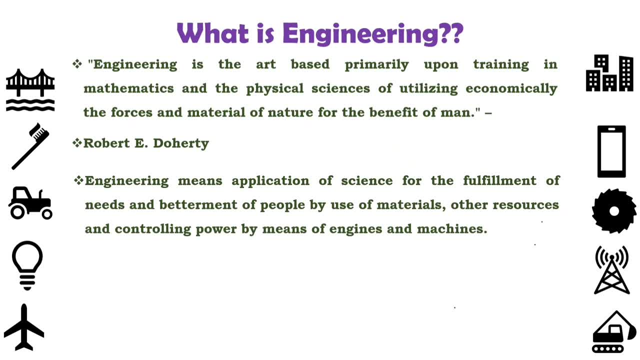 Engineering means application of science for fulfillment of need and betterment of man, The use of people by use of material other resources and controlling power by means of engines and machines. We can also say engineering is concerned mainly with the designing, fabricating, erecting, manufacturing, installing, operating, controlling and maintaining engines, machines, instruments and equipment. 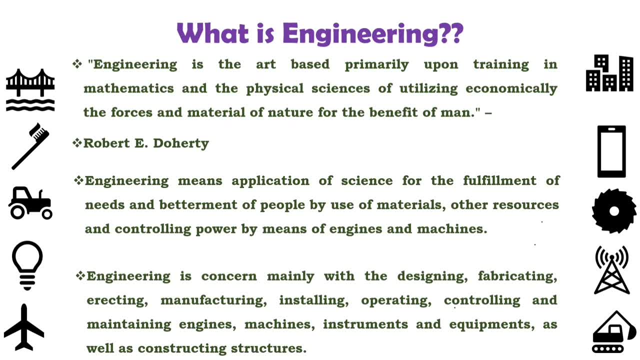 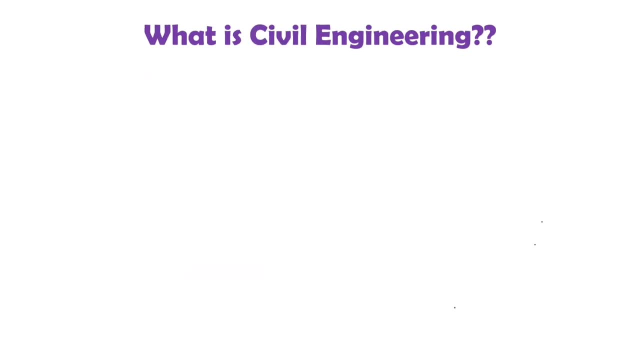 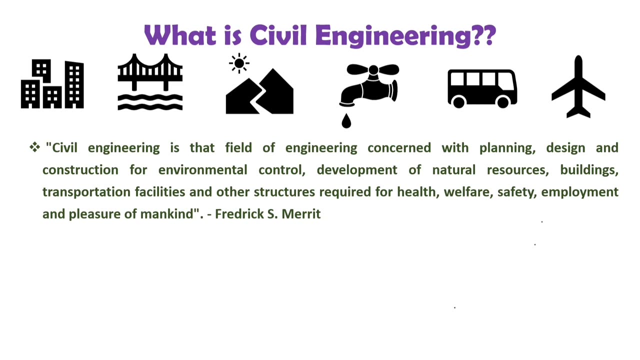 as well as constructing the structures. So we can say engineering is the science of fulfillment of, or we can say betterment of, people. Now let us say what is civil engineering? Civil engineering is that field of engineering that concerned with planning, design and construction of environment control. 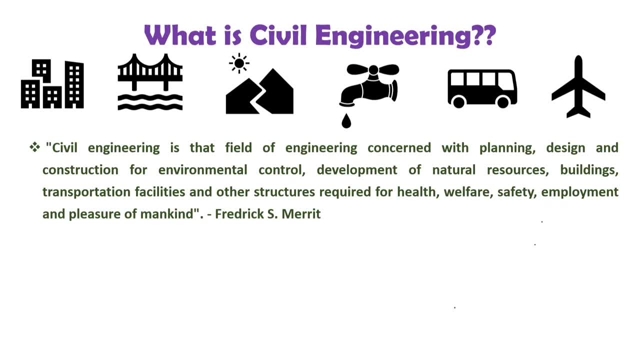 development of natural resources, buildings, transportation facility and other structures required for health, welfare, safety, employment and pleasure of mankind. This is the statement by Frederick S Merritt: Civil engineering can be designed to fulfill the needs of all people. Civil engineering can be. 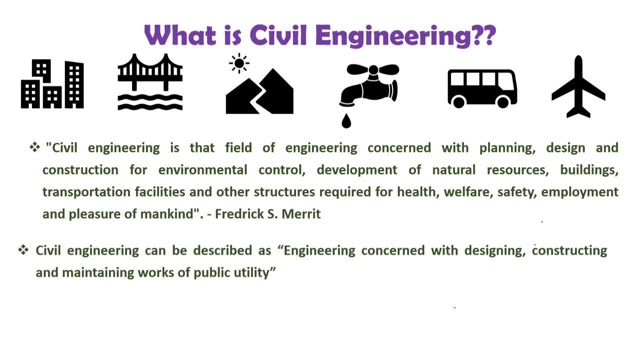 designed to fulfill the needs of all people. Civil engineering can be described as engineering concern with designing, constructing and maintaining works of public utility. Civil engineering is that branch of engineering professionals which deal with planning, designing and construction of structures. Basically, civil engineering is related to civilians. That's why it is called 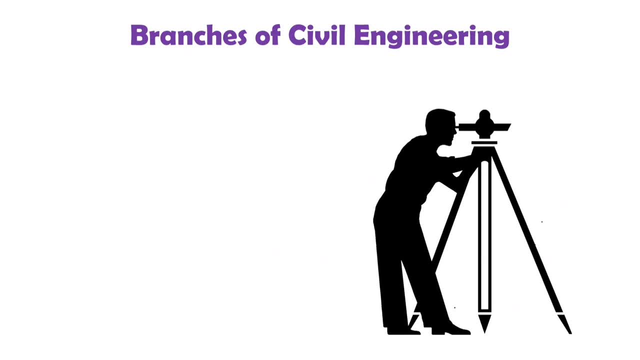